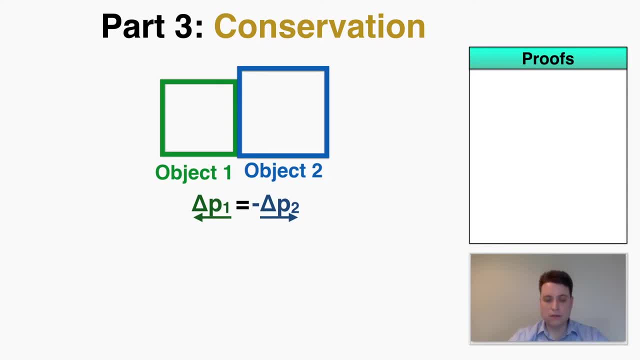 experiences impulse, the other object always has to experience the exact same amount of impulse, but in the opposite direction. So that's an interesting concept and we can draw out a little more info from that idea. Just as an example of what this would look like, let's say that we have 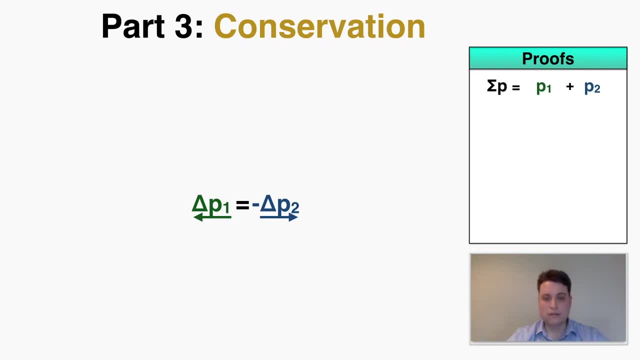 two objects moving toward each other with negative 10 Newton seconds. I'm considering right to be negative and left to be negative, So I'm going to draw out an example of what this would look like. I'm going to set the pulse to be positive and 20 Newton seconds, like this, And I'm going to use a new concept. 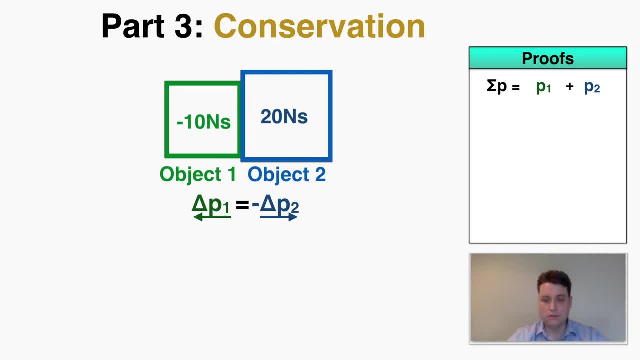 up in the proofs box. and now, considering the total momentum of the system, I want you to observe something about the total momentum of the two objects added together. So I can see that I'm starting with a momentum of negative 10 and a momentum of positive 20, so that means that the 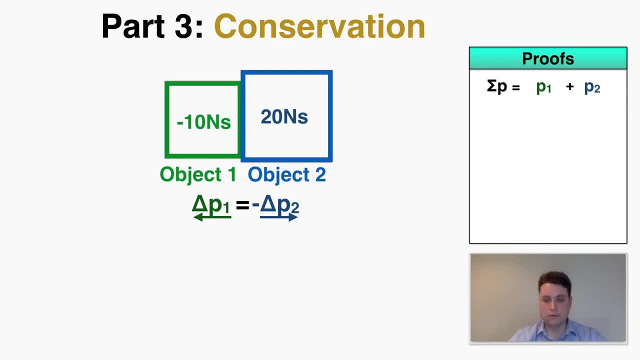 total momentum between these two blocks, if I add both of those together, is going to be 10 Newton seconds of momentum, negative 10 plus positive 20.. I'm now going to imagine that object 1 experiences an impulse of 30 newtons to the left and 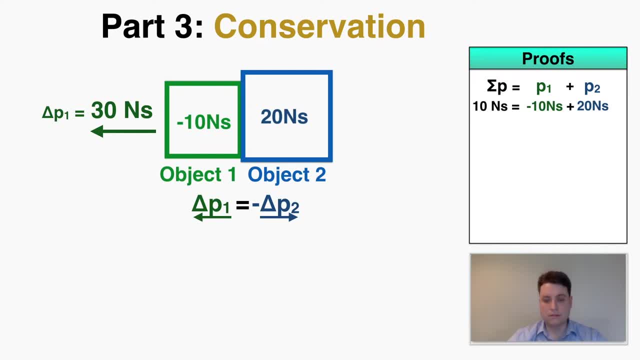 I'm considering left to be positive, so that's a positive impulse. So, based on the idea that I just showed you in the previous slides, if that object 1 is experiencing a leftward impulse of 30 newton seconds, that means that object 2 is experiencing. 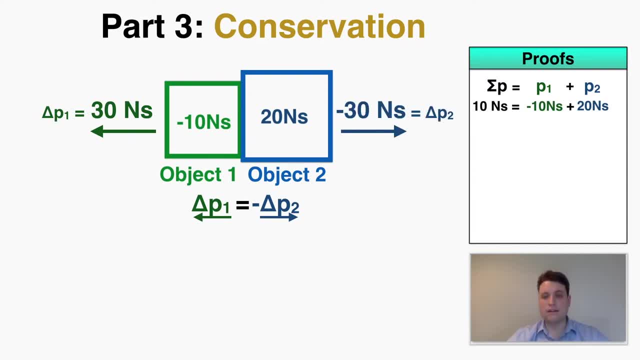 a rightward impulse of 30 newton seconds, so I'll consider that negative. So, remembering now that impulse is not just the force times, the time, it's also equal to the change in momentum on the object. So this means that object 1's momentum is changing by positive 30 newton seconds and 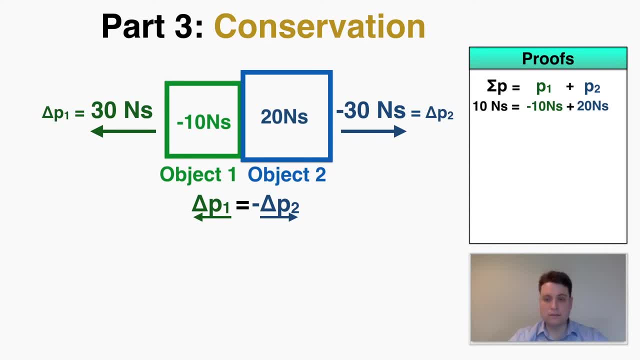 object 2's momentum is changing by negative 30 newton seconds. So when I add these two changes to the two objects, I get a final momentum of 20 newton seconds on object 1, and a final momentum of negative 10 newton seconds on object 2.. 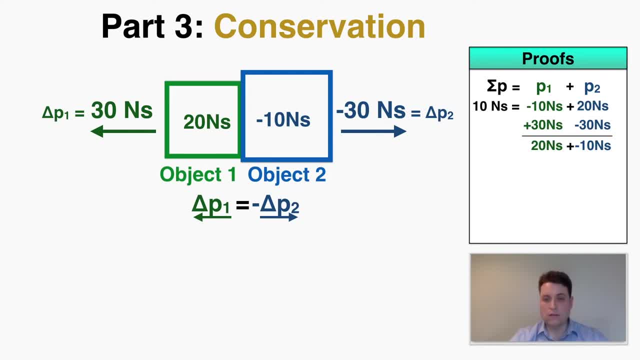 I added 30 to object 1, and I took away 30 on object 2.. So you'll notice that the two individual objects now have new inputs, But if we consider the total momentum between them, like the total momentum in this system. 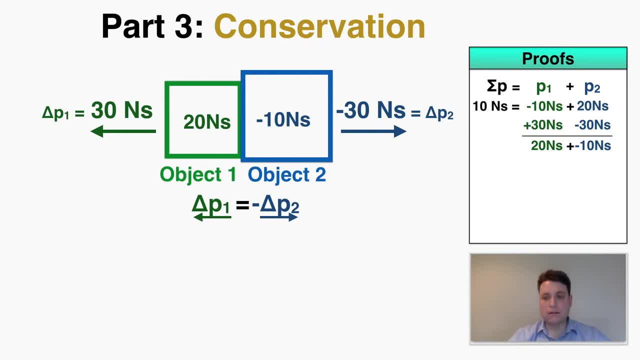 I added 30 newton seconds on one side, but I subtracted it on the other side. So that means that the total momentum didn't change in that situation- and I can see that it didn't- The total momentum is still positive 10.. 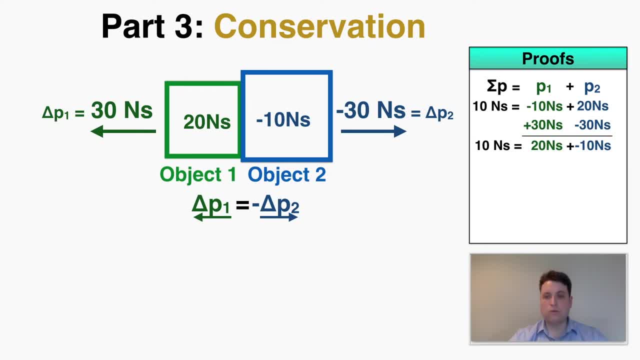 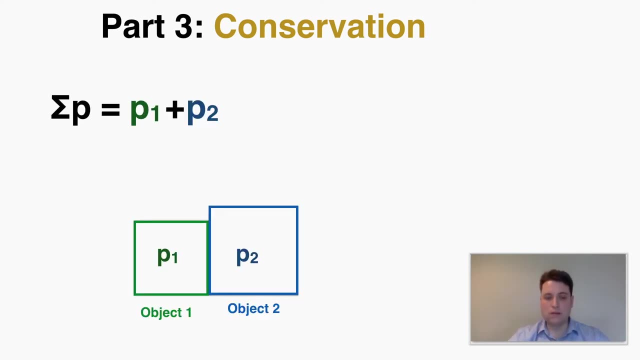 The individual momentums of the objects changed, but the total remained the same. It stayed at positive 10.. This rule about the total momentum staying the same whenever two objects put a force on each other can actually never, ever be broken. You'll notice that no matter what impulse I choose to put on object 1, object 2 is always. 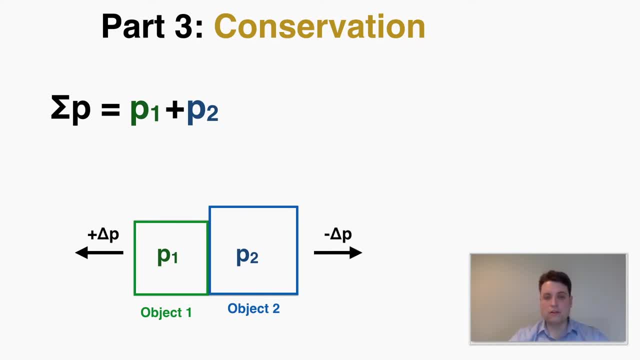 going to experience that same impulse, but in the opposite direction, so it'll be negative. So whatever I add to object 1, I have to take away from object 2. And if I plug both of those into my equation for the total momentum, they're both cancelled. 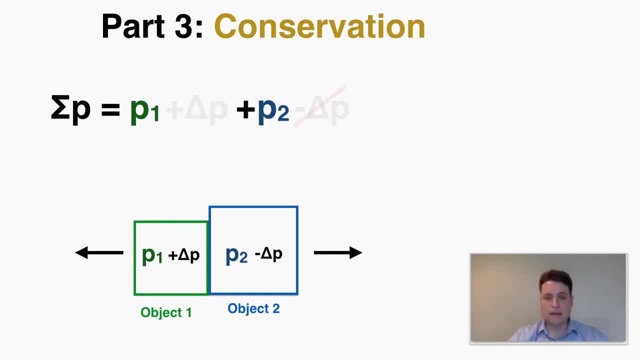 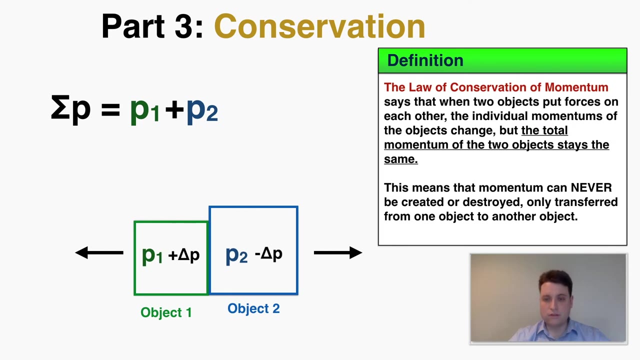 out, And so the total momentum is always going to remain at that same total amount that it started with, As long as those two objects stay the same. So this leads to a new definition. This is the law of conservation of momentum. The law of conservation of momentum says that when two objects put forces on each other, 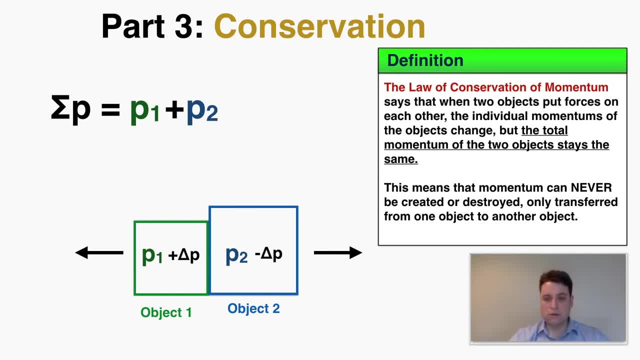 the individual momentums of the objects change, but the total momentum of the two objects stays the same. This happens every single time two objects interact with each other. The two individual momentums of the objects can change, but there's some the two momentums. 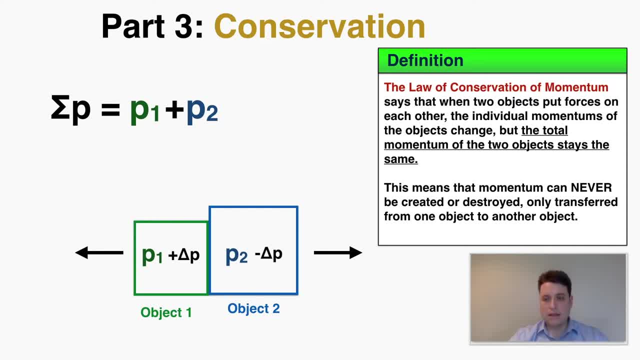 added together stays exactly the same, And the implication of this is that momentum can never possibly be created or destroyed. Momentum can never come into or leave the universe as a whole. It can only be moved around from one object to another object. One implication of this, which is pretty crazy, is that the universe has never gained or lost. 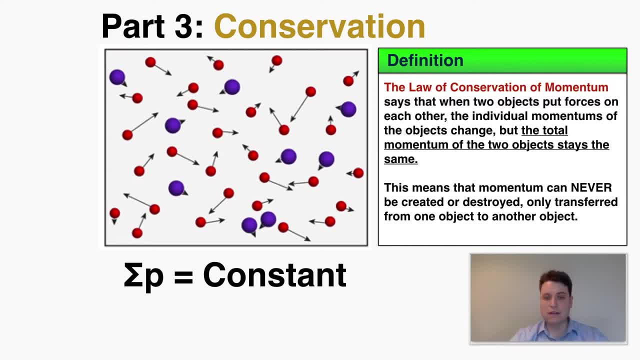 any momentum ever, The total momentum in the universe added together. if you were to add together every single mass times velocity of every single particle, that would be the total momentum of the universe. That would be the total mass times velocity of every single particle. that would be the 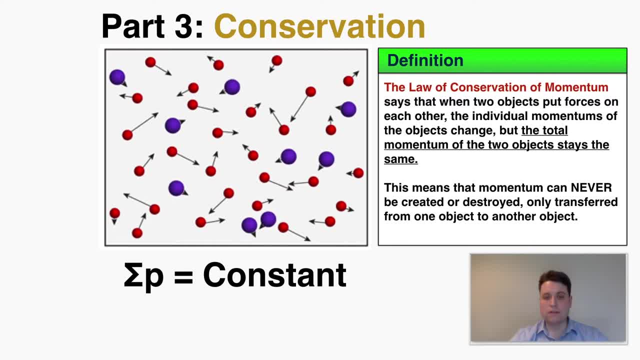 total mass times, velocity of every single particle in the universe. That total momentum would be some constant, which is pretty incredible to think about. The momentum can't possibly be gained or lost in any way, So this seems like it would probably have a lot of predictive power for understanding. 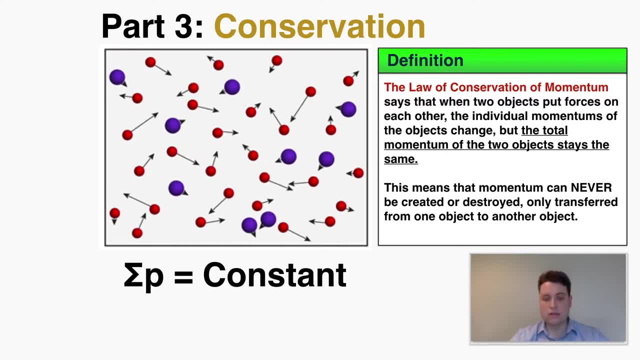 how objects are going to move in the future. if this value isn't changing- And that's true- it does have a ton of predictive power. The reason why we care so much about conservation is that, using this idea that the total stays the same, we can predict a lot of new information about objects that are interacting with each other. 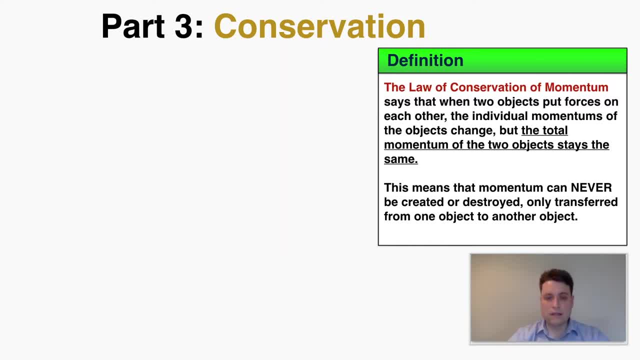 In general, a quantity that is conserved can never be created or destroyed, only transferred or transformed into another type of that same quantity. There are a few different things that are conserved. in physics, Things like momentum, energy, mass and electric charge are all conserved. 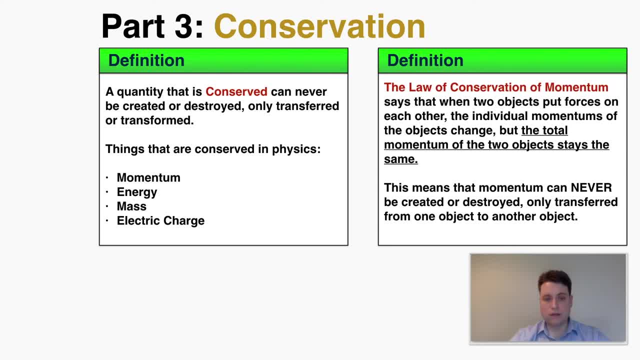 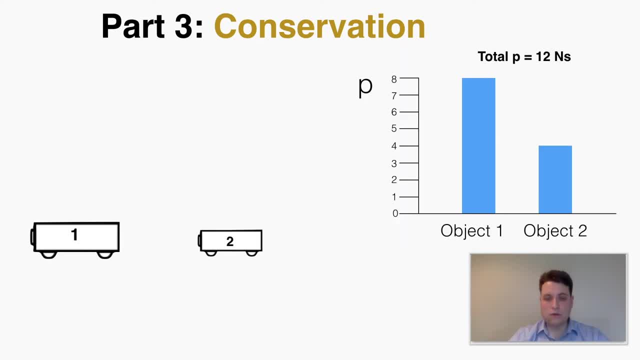 So none of these things can ever be created or destroyed, only transferred or transformed. Just as an example of what this looks like in problem solving, we can imagine that we have two carts. One is moving in the same direction, but the cart number 1, object 1, has more momentum. 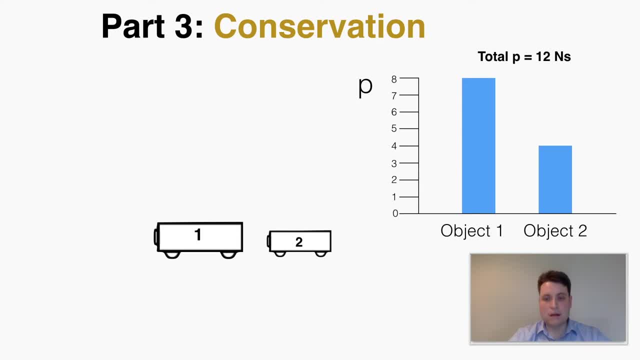 than object 2.. I'm going to use this graph above my head to say that object 1 has 8 newton seconds of momentum and object 2 has 4 newton seconds of momentum, so the total is going to be 12.. 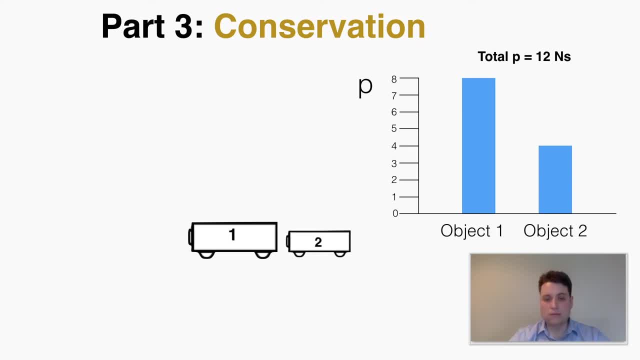 We can now imagine that they have some impact at some point. So object 1 impacts object 2 and puts some impulse on it. So whatever impulse object 1 gives to object 2, object 2 gives back to object 1.. So object 2 is going to gain that rightward momentum, whereas object 1 is going to lose. 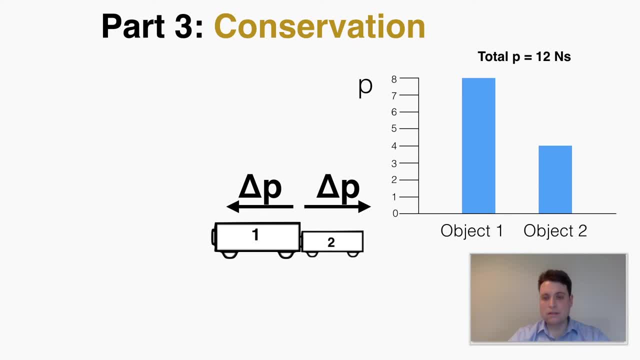 that rightward momentum or gain leftward momentum. So basically, looking up at my graph, that's basically object 1 giving a chunk of its momentum, this change in momentum over to object 2. So when that happens, the total remains the same. 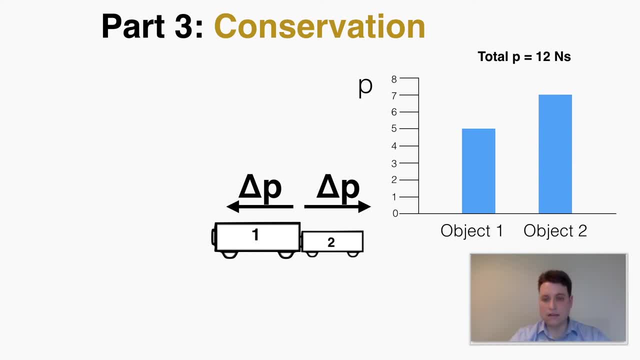 The total amount of momentum that the two carts have has stayed exactly the same. It's remained at 12.. But now cart 2 has more momentum than it had before And cart 1 has less momentum than it had before. So they might move off like this. 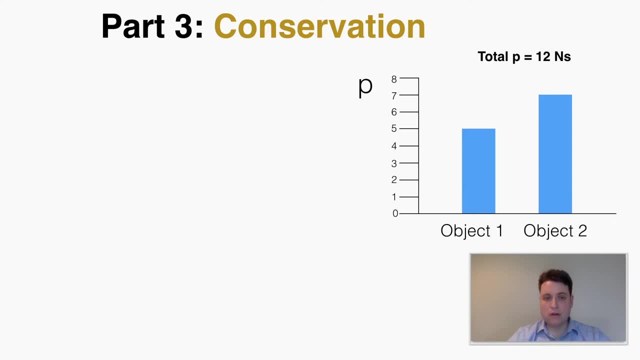 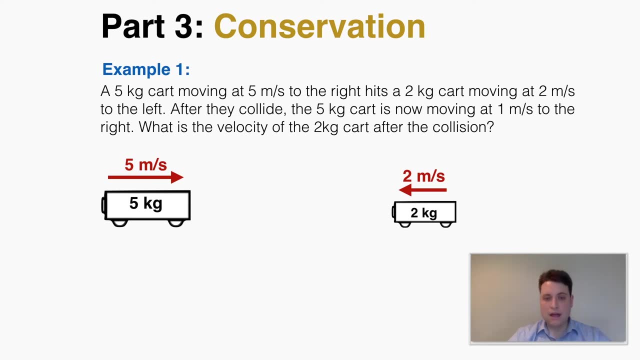 We can now do some examples with actual numbers. For example, a 5-kilogram cart moving at 5 meters per second to the right hits a 2-kilogram cart moving at 2 meters per second to the left. After they collide, the 5-kilogram cart is now moving at 1 meter per second to the right. 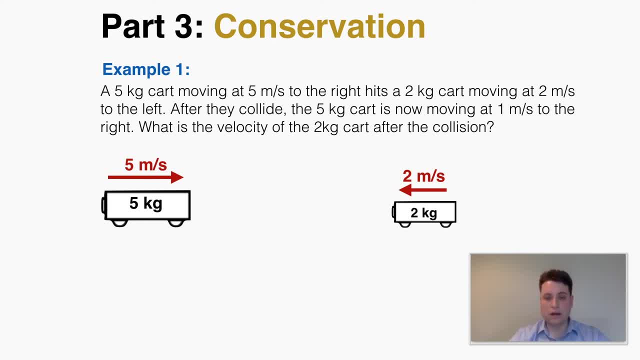 What is the new velocity after the collision of the 2-kilogram cart, after the collision? So I'm going to start by defining directions. I'm going to say right is positive and left is negative And when these two carts collide, the total momentum in the system is the momentum of 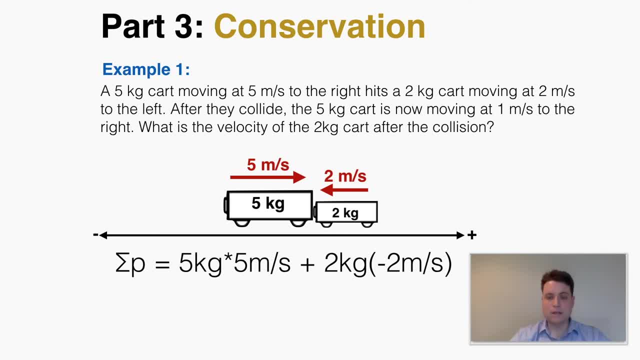 the cart moving to the right, which is its mass times its velocity, which is 5 times 5, plus the momentum of the cart moving to the left, which is its mass, 2 kilograms times its velocity, which is negative 2 meters per second because it's moving in the negative. 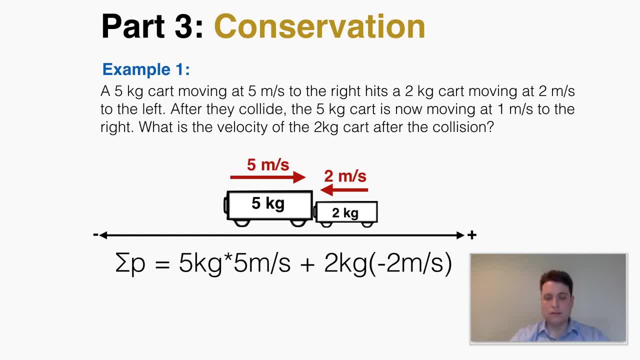 direction, And when I add these together I get a total momentum of positive 21 Newton seconds. That's how much total momentum is in this system. So the problem says that after they collide, the 5-kilogram cart is now moving at 1 meter. 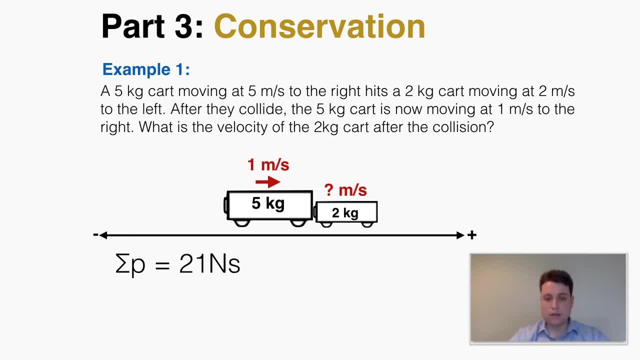 per second to the right and we want to know the velocity of the 2-kilogram cart. So, plugging this in, adding those two new momentums together, I know that the total momentum is going to stay the same. So the momentums of these two carts added together is going to equal 21 Newton seconds. 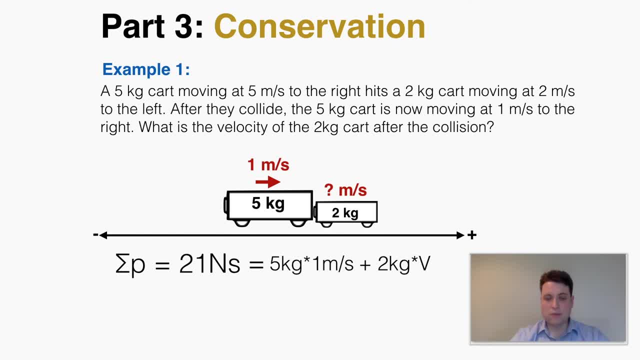 So the new momentum of the 5-kilogram cart is 5 kilograms times positive 1 meters per second. The new momentum of the 2-kilogram cart is 2 kilograms times that new velocity that we're solving for. And now I can just use algebra to solve for velocity by itself and I get 8 meters per. 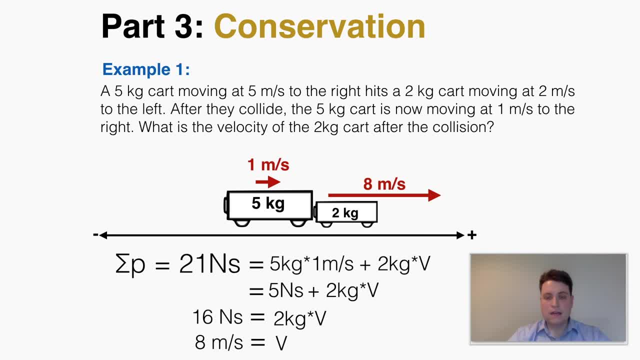 second. So that means that after these two carts collide, it's 100% certain that if the 5-kilogram cart is moving at 1 meter per second, the 2-kilogram cart is going to be moving at 8 meters per. 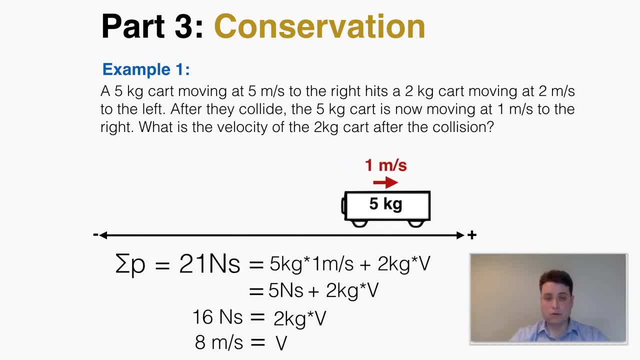 second like this after the collision. So we're 100% certain of that, based on the laws of physics that we know already. Here's one more example of conservation. We can now imagine that a 5-kilogram cart is moving at 2 meters per second when we drop. 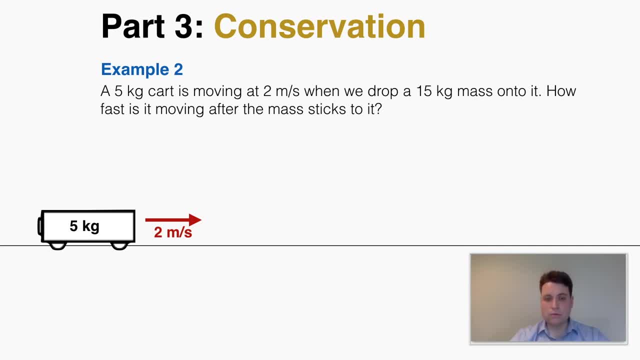 a 15-kilogram mass onto it, and how fast will it be moving after the mass sticks to the cart? So, as this is moving, it starts off with a total momentum of 5 kilograms times 2 meters per second. There's no additional momentum in the system right now. 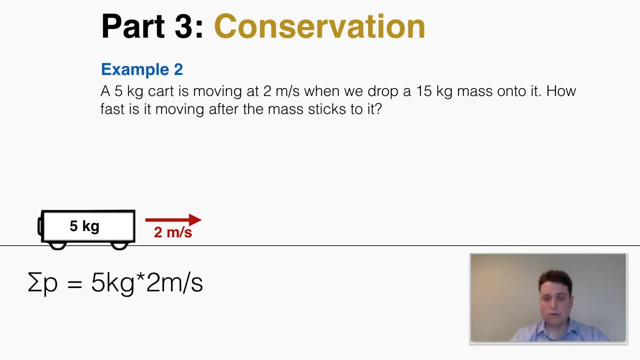 It's just the cart moving to the right. We're now going to imagine that we drop a box onto it, that's 15 kilograms, and you'll notice that when the 15 kilograms hits the cart, Something kind of weird happens, where, because the downward force of the box is balanced,